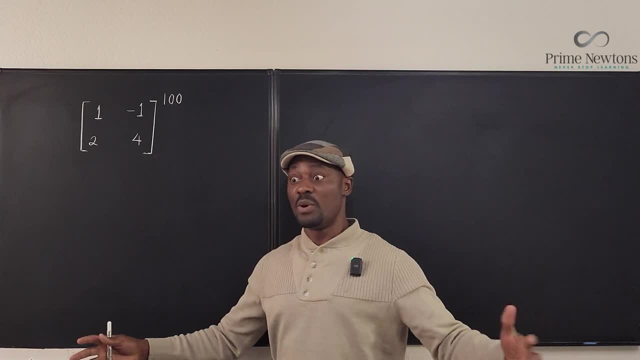 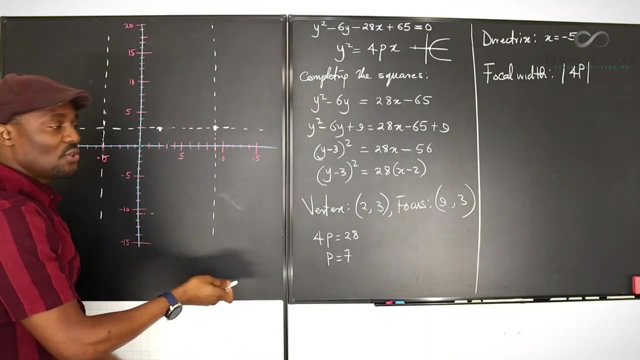 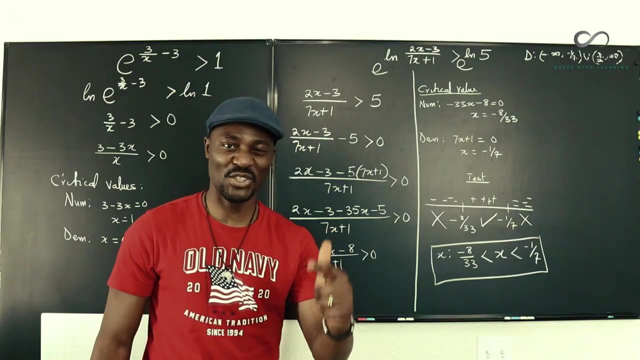 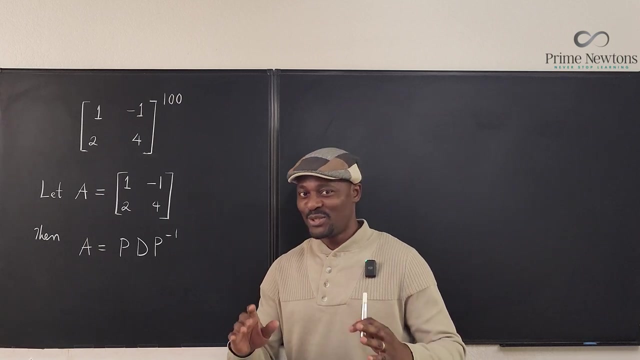 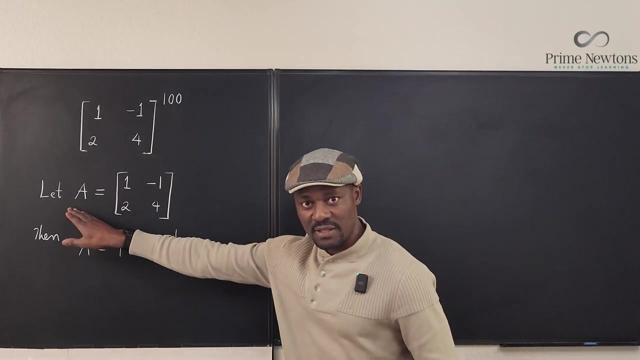 and raising a matrix to the super big power. Let's get into it. So this is the secret to diagonalization. It is not complicated, okay, Because this topic could be somehow confusing, but do not confuse yourself. Any matrix, if it is diagonalizable, can be. 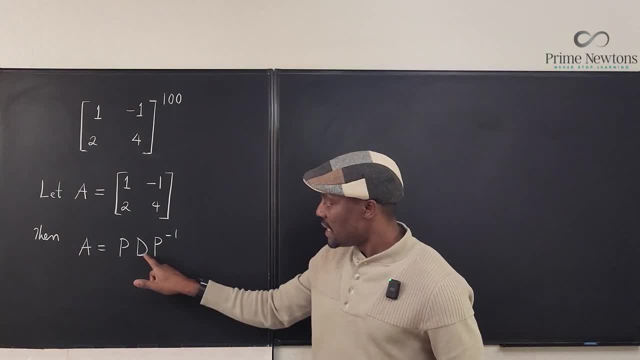 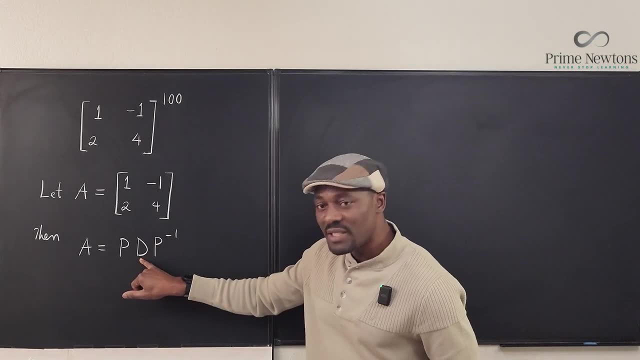 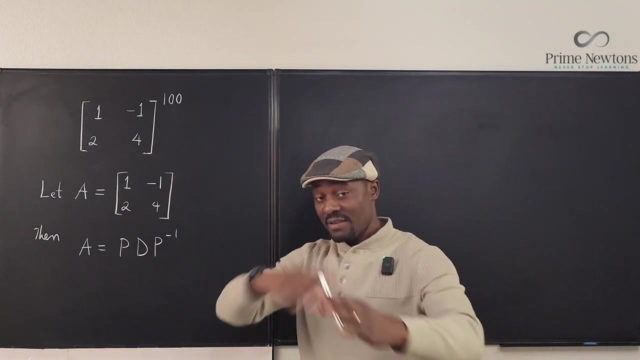 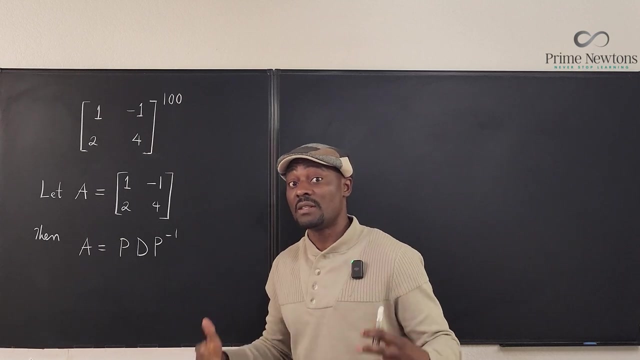 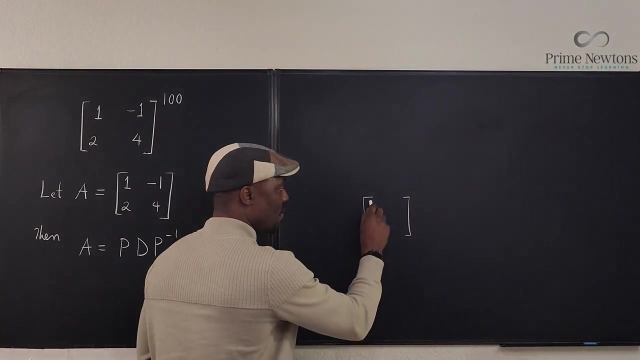 written as PDPX. And what does that mean? It means you see, this matrix in the middle is a diagonal matrix, And what that means is that every entry in the matrix is zero, except on the main diagonal. That's where you're going to find entries that are not zero. So, for example, if I write a matrix say 1, 0, 0,, 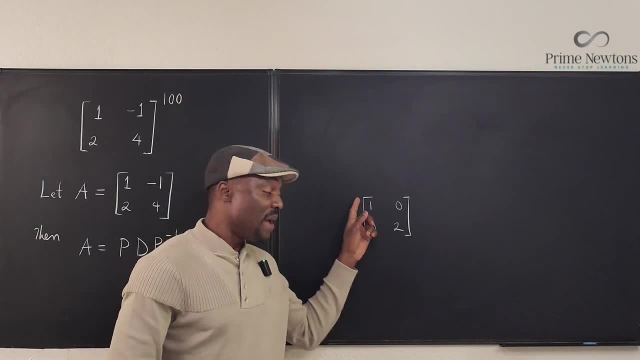 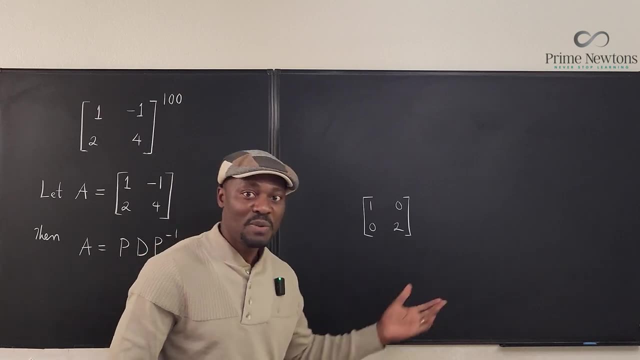 2,. this is a diagonal matrix Because on the main diagonal you have the non-zero entries. Everywhere else you're going to get zero. So, whether it's a 2x2 or a 3x3, I'm using a simplified version. 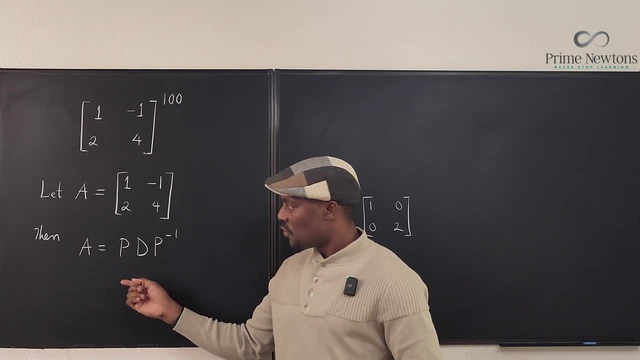 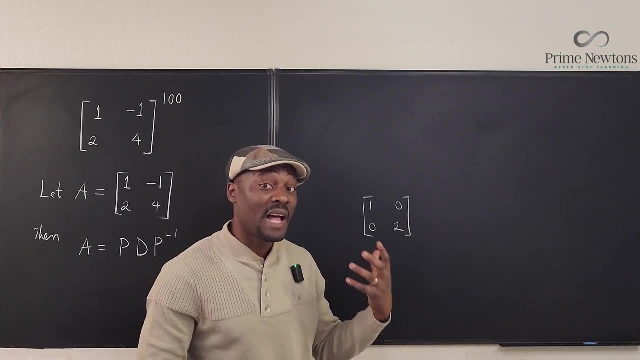 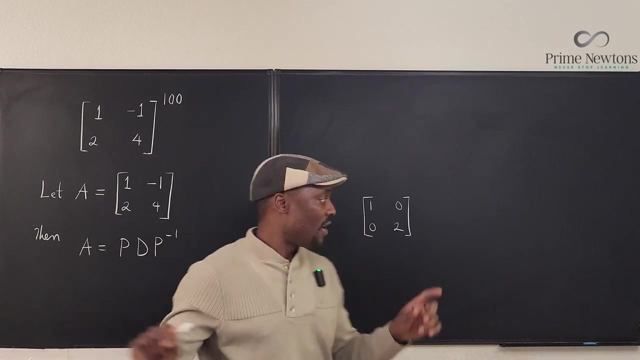 Now, if we are doing this, you're going to ask me: so, if this is D, how do I get these numbers? Well, these numbers are those eigenvalues that you get from the computation. okay, So the eigenvalues of this matrix A are what you're going to put on the diagonal. Now, how do I know which one? 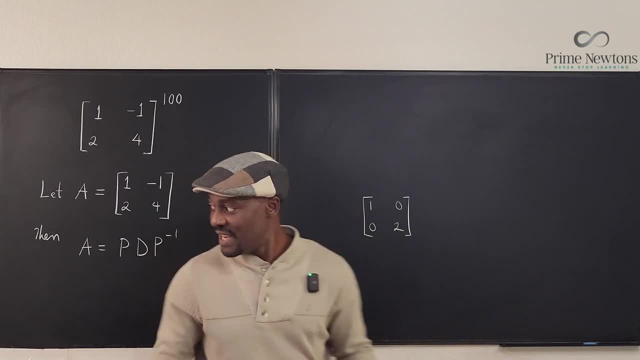 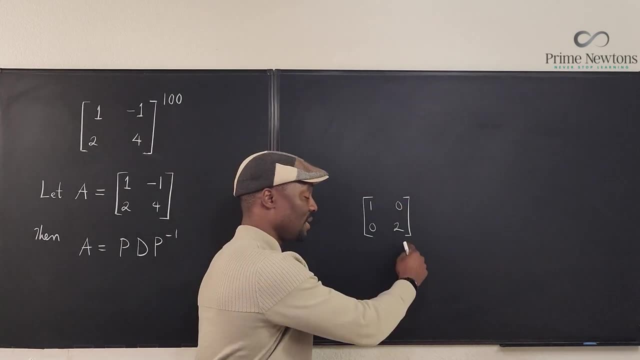 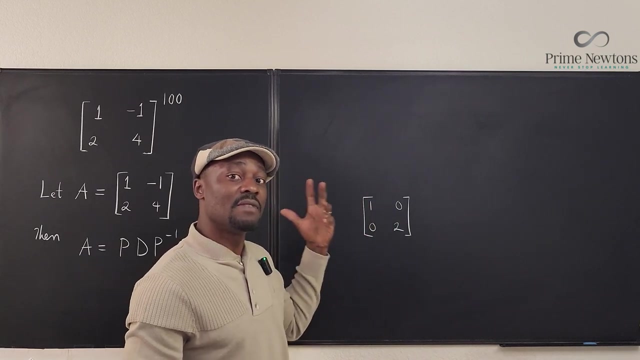 comes first. It doesn't matter, okay, Because the D that you have is not unique. okay, You can switch them. You can put this 2 here, put this here. The only thing is, whatever eigenvalue you put here, the column must correspond to the eigenvector, that is. 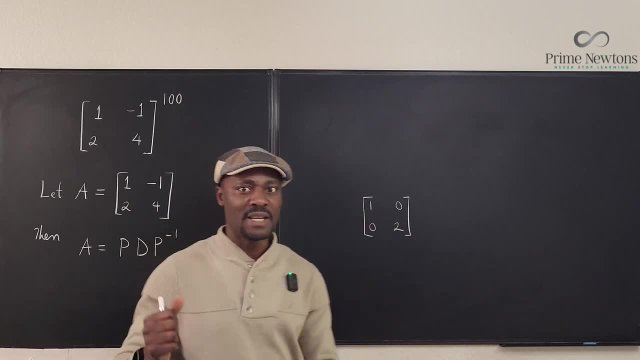 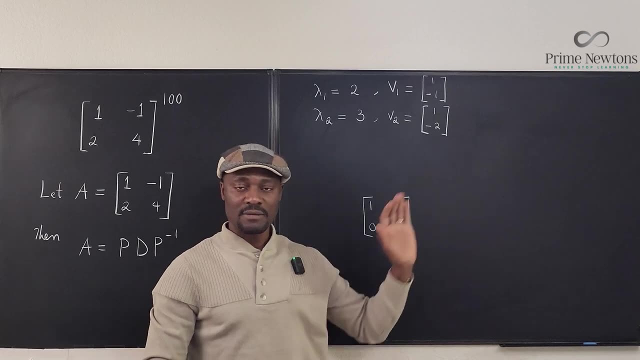 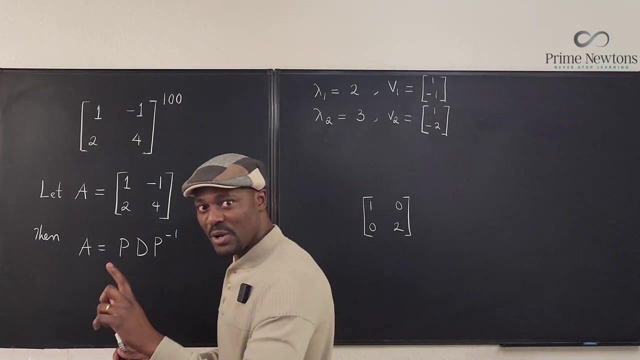 corresponding to that eigenvalue. So I remember that when I did this video before, I got the result for the eigenvalues. so these were: this is all I need. so all I have to do is create this environment. so watch what I'm going to do, because these are all. 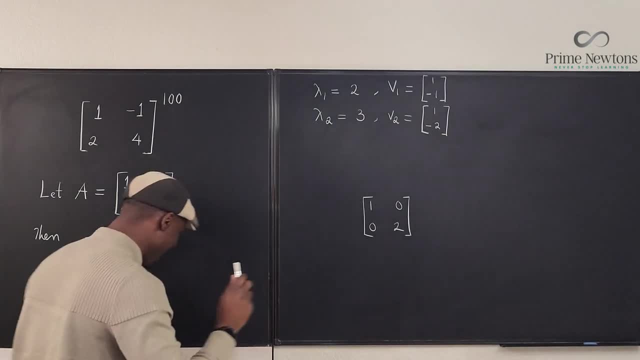 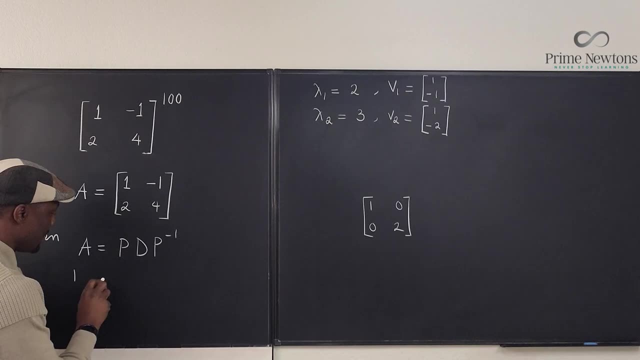 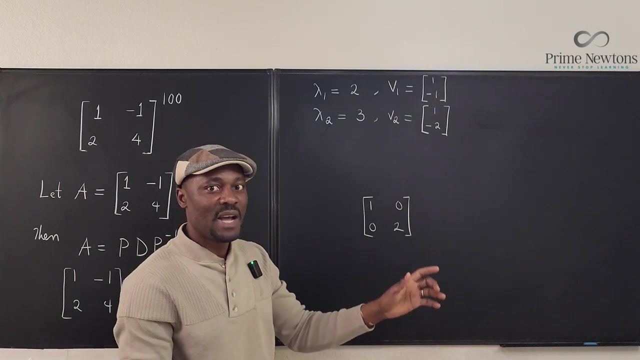 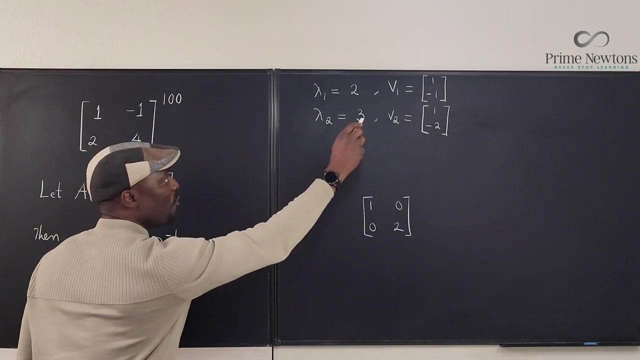 the four things you need. okay, so watch this. my matrix a, which is 1, negative, 1, 2 & 4 can be written. as you see, the P here is a stack of these two. just put them side by side inside the matrix. so this is P, right here it's gonna be 1. 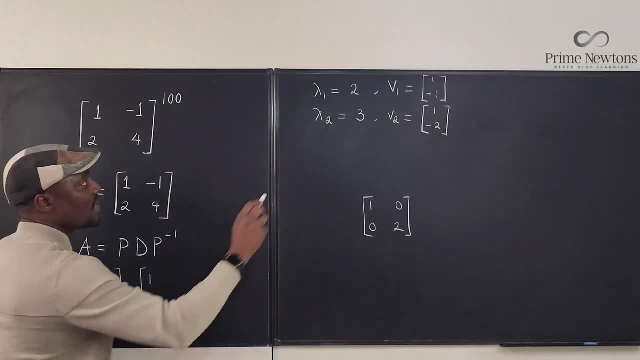 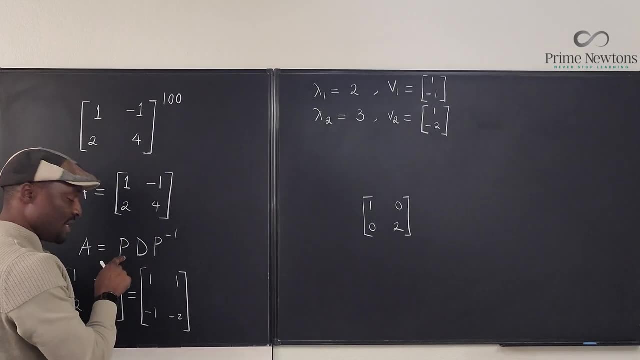 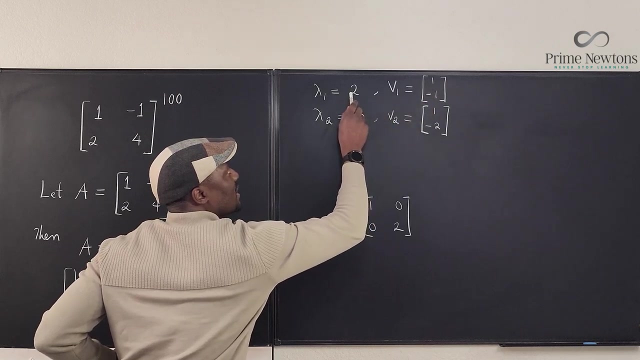 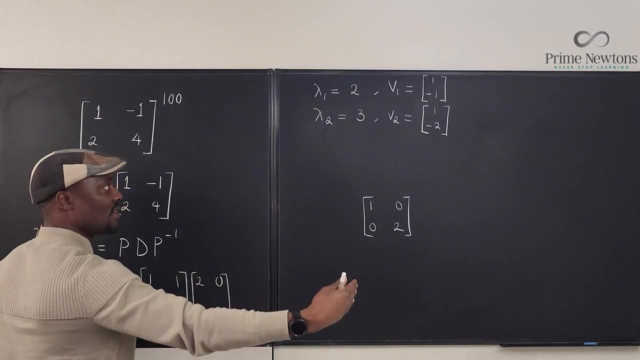 minus 1 and the other is 1 minus 2. that's P. what is D? it's the easiest and the nicest thing it is. remember I told you you just need these two. so because I put this on the left, it is corresponding to this. so I'm going to put this two here. and because I put this on the right, 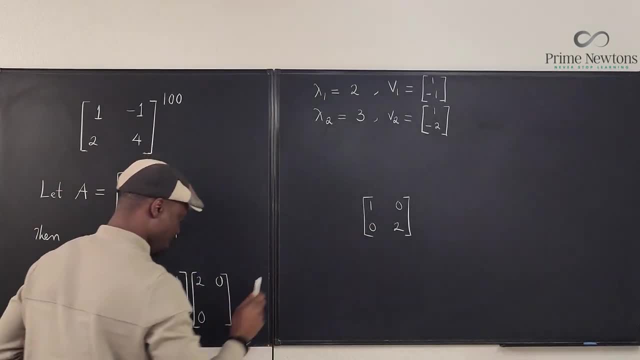 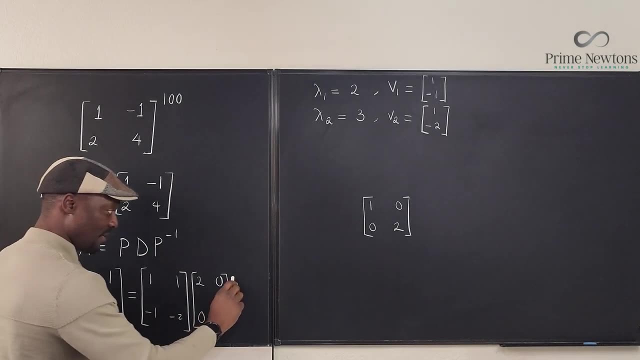 the 1 negative 2, which corresponds to this. I'm gonna put this 3 here now. okay, tell me, what am I gonna put? what is this one? well, it is the inverse of P. this is narrow, okay, I'm gonna manage it there, and this is gonna be 1, 1 minus 1 minus 2. 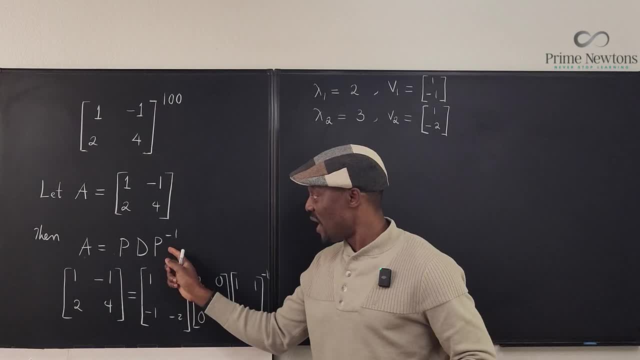 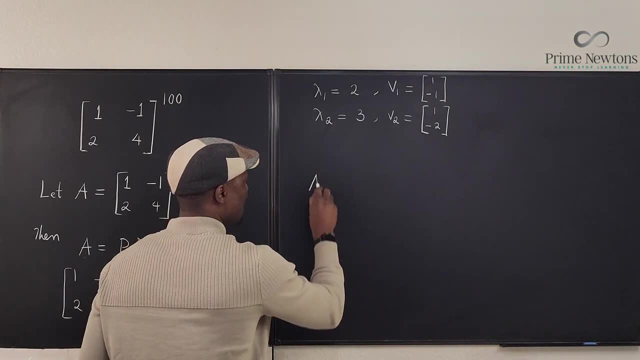 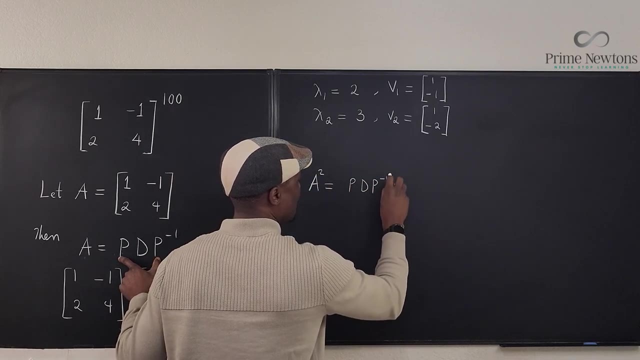 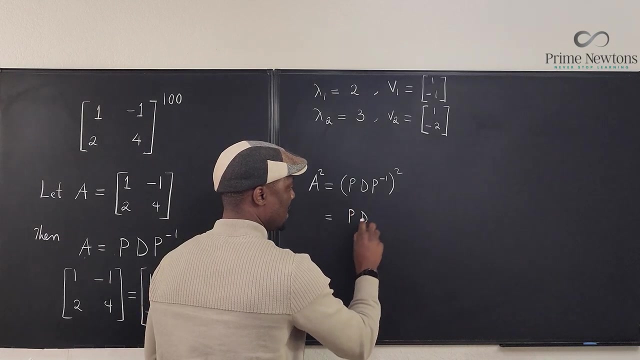 that's it. so let me quickly explain how this one, raised to the power 100, is gonna work. let's just do power 2. let's do power 2, okay. so look, a squared is gonna be this square. it's gonna be P D P- inverse square. but you see, this can be written as P D P. 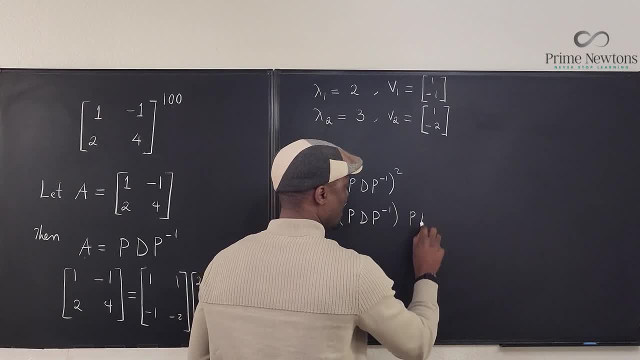 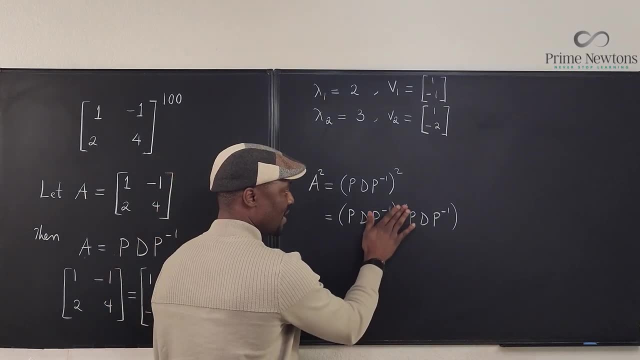 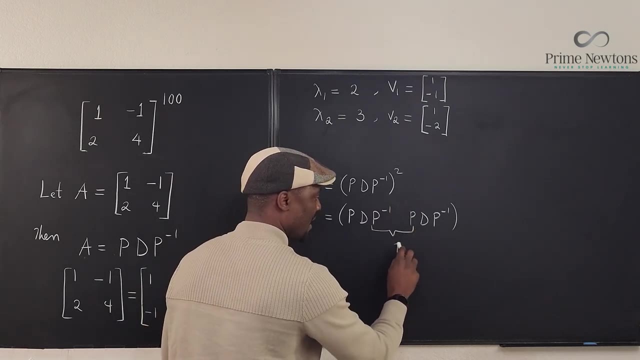 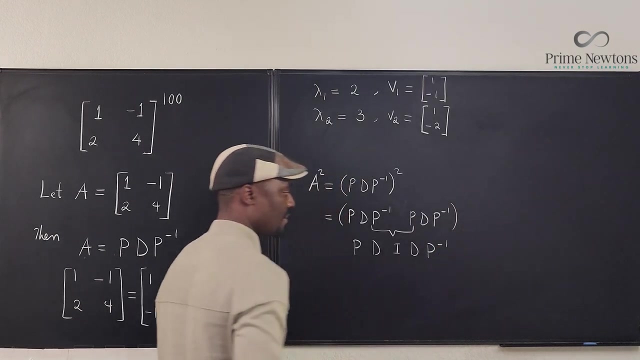 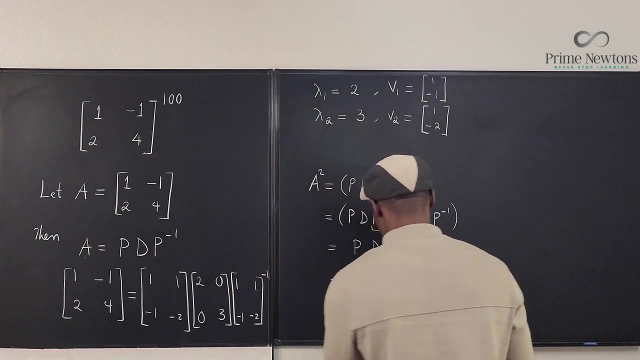 inverse times P D, P inverse. now, if we remove the parenthesis and we stop multiplying, you see P times its own inverse is just I. that's P times D times I times D times P inverse. well, D times I times D is just D squared. you see that what has just happened is we have squared just. 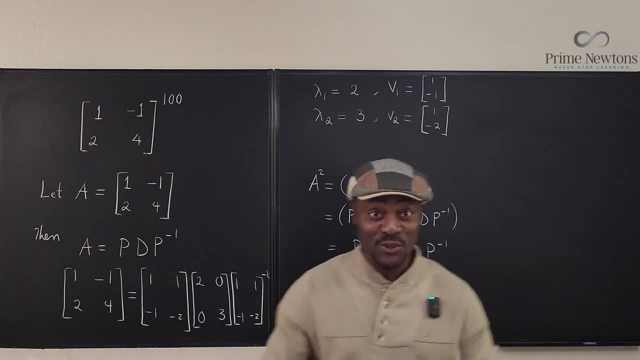 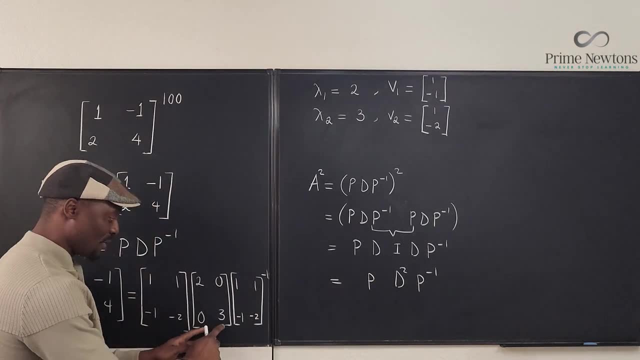 the diagonal matrix. and it's always easy to square a diagonal matrix because all you have to do is go to the diagonal matrix and this value means that at the the diagonal, where is it? if you want to multiply this matrix by itself, all you're doing is just 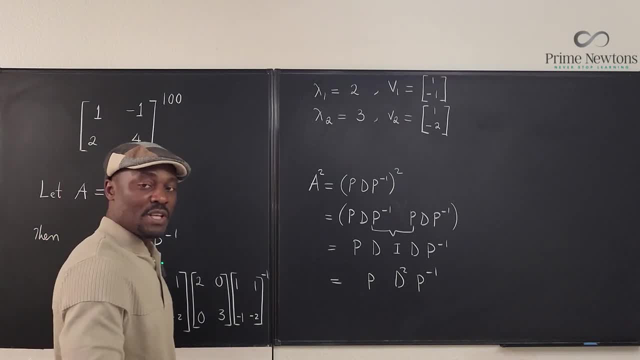 squaring this and squaring this. if you, if you raise it to power 10, you just raise this to power 10. raise this to power 10, because if you try to multiply this by itself 10 times, you'll find out that all you're doing is you're raising. you just keep multiplying this by itself and multiplying. 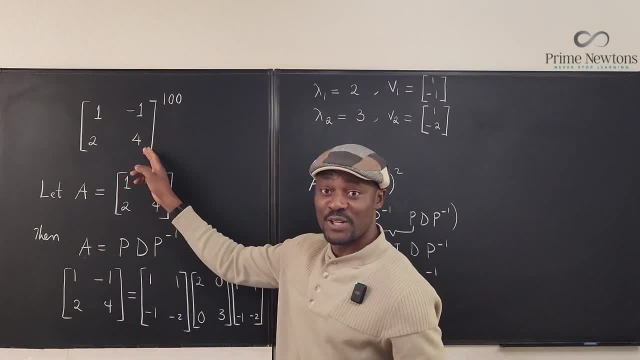 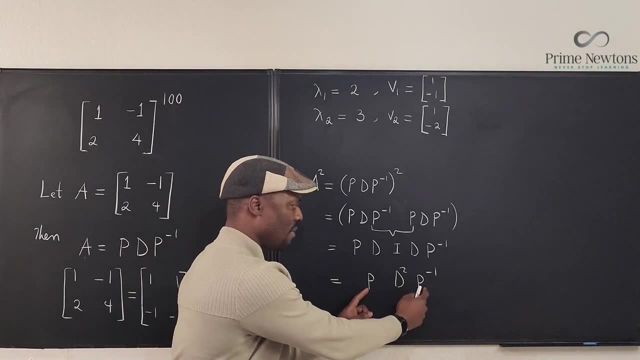 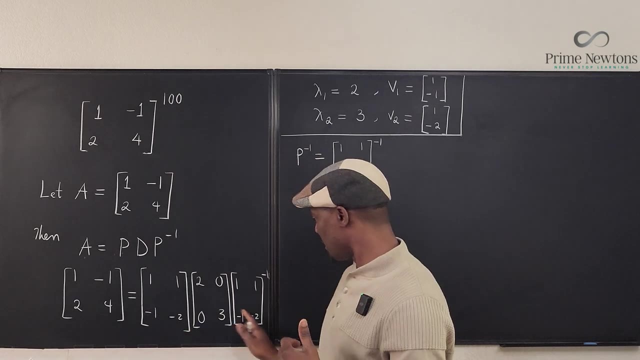 this by itself, and that's why it is possible to do what we're going to do here: to raise it to power 100. so after raising this to its, the power you want, you can then multiply by just these two basic matrices. let's quickly compute p inverse, because we'll need it for this final calculation. let's 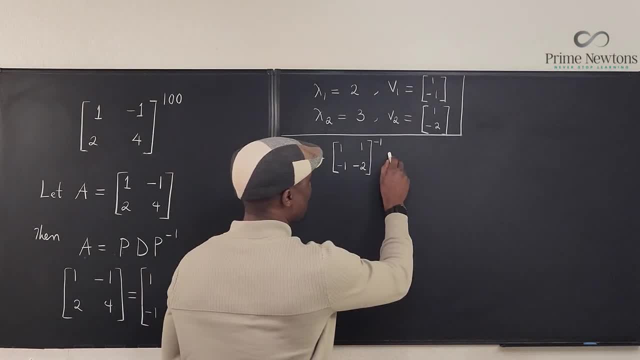 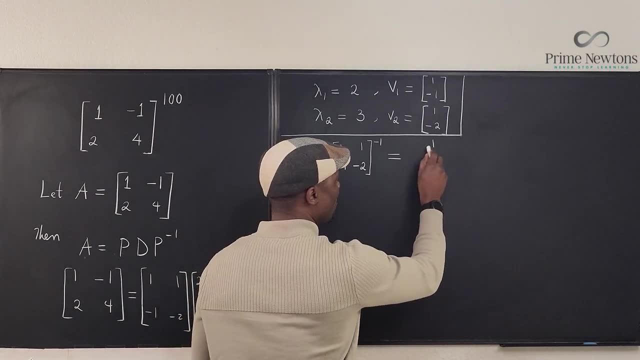 know what this is. so here, this is going to be equal to. well, let's use our shortcut method. what's the inverse of a two by two matrix? it's going to be one over the determinant of the matrix. what was the determinant of this? so it's going to be: 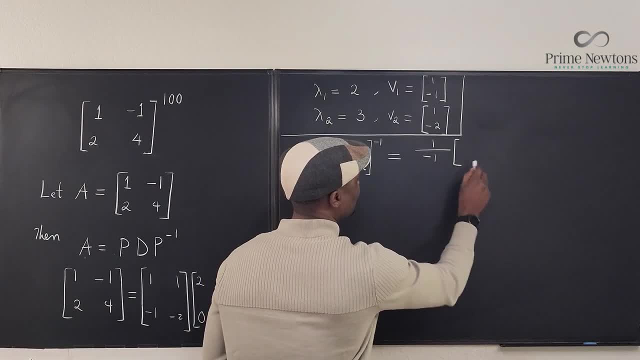 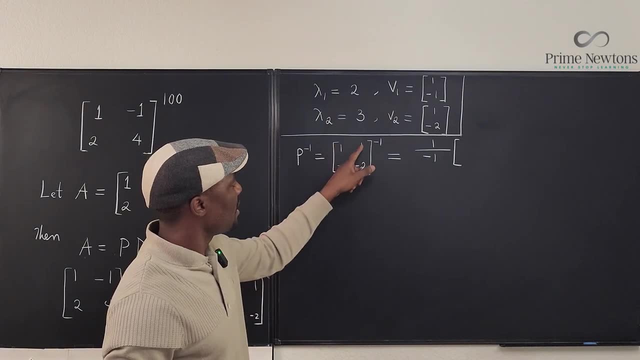 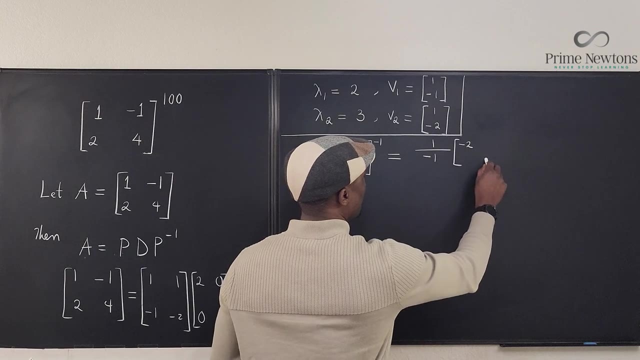 one over negative one times. well, we're going to get the adjoint of this. the adjoint of this is going to be: we're going to switch these two and change the signs here. so this is going to be minus two and this is going to be um one, and then we're going to switch the signs here. this is going to be. 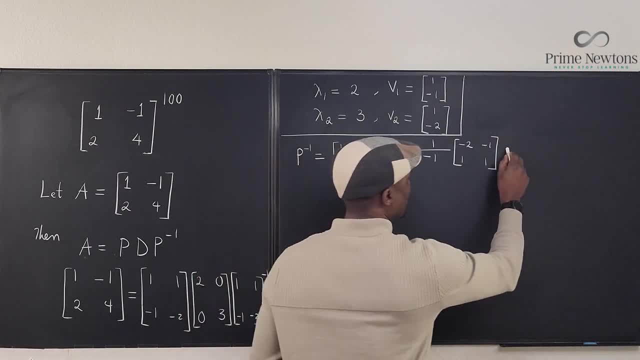 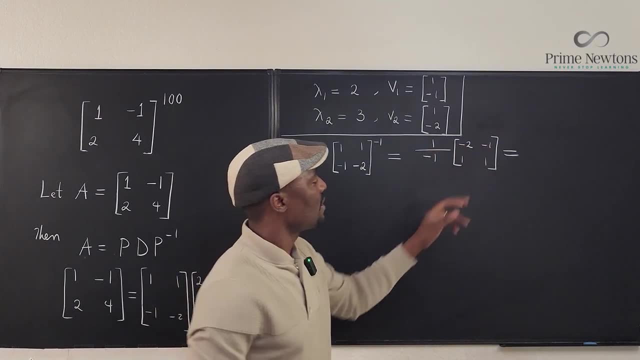 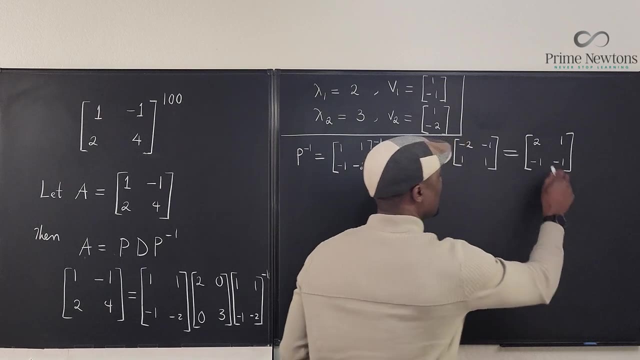 one and this minus one. okay, and what does that give us? let's just go this way. well, this is going to be minus one times this, so this is two, two minus one, and this is going to be minus one and minus 1, minus 1.. So it's going to be 2, sorry, 2, 1, minus 1, minus 1.. Okay, we've gotten our. 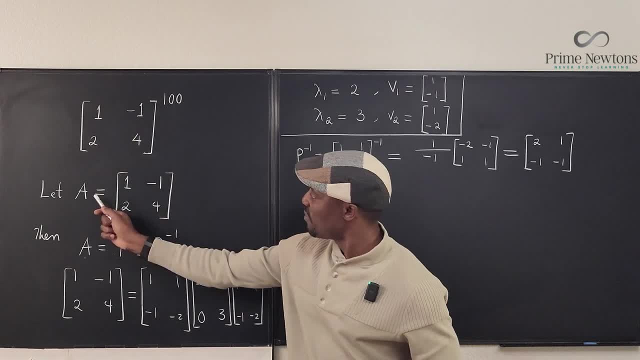 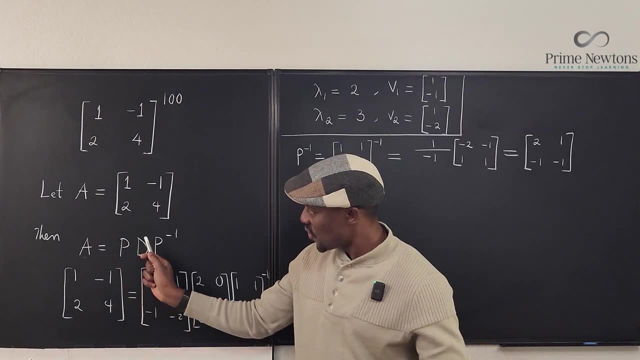 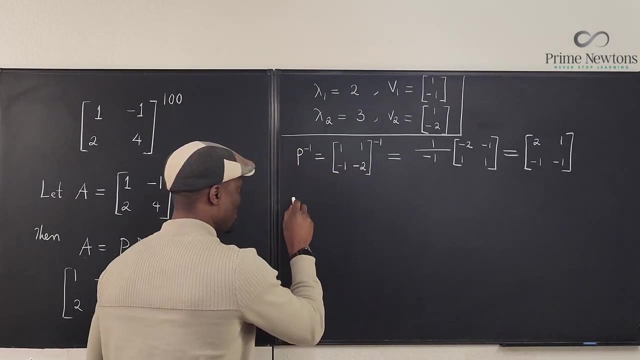 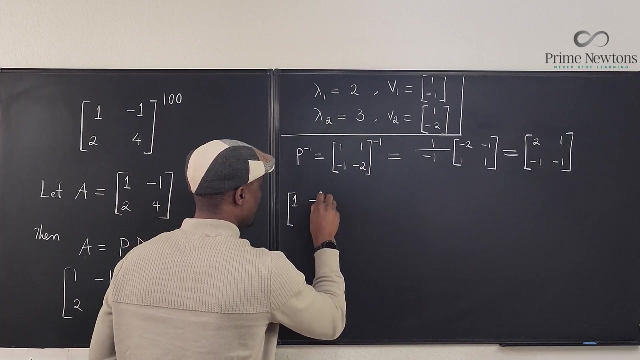 inverse. At this point, I need to raise this to power 100, which means I need to raise this to power 100. And, like I explained, you only need to raise this to power 100, and we already know what this is going to be. So let's write this. So we have this, which is 1, negative, 1, 2, 4.. Raise to. 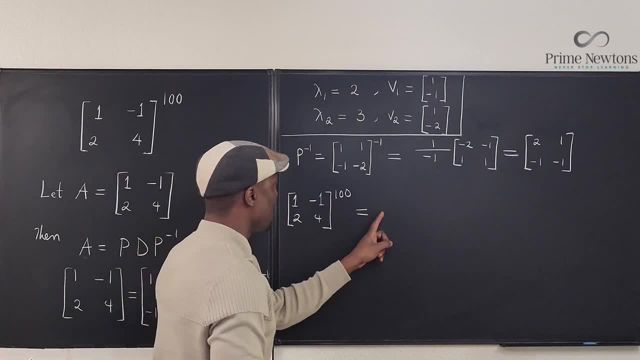 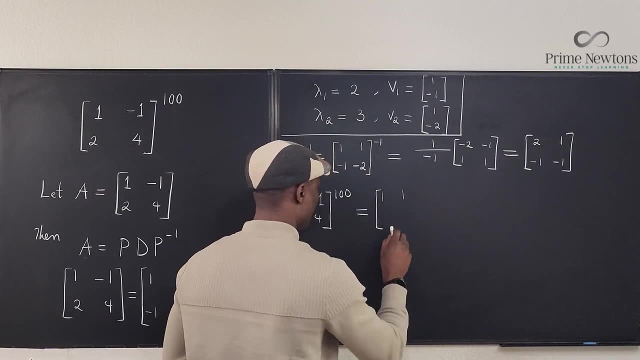 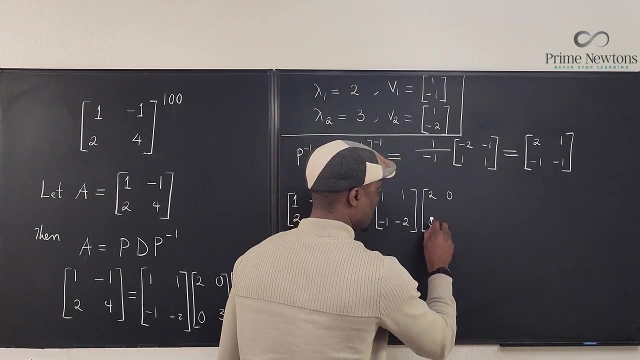 power 100 is equal to P, which is this: 1, 1,, 1, 1, negative, 1, negative 2.. Times the diagonal matrix, which is the matrix of just 2, 0,, 0,, 3,, 2,, 0,, 0, 3, raise to power 100,. 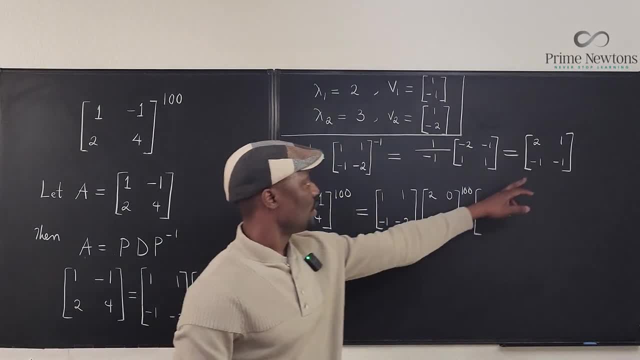 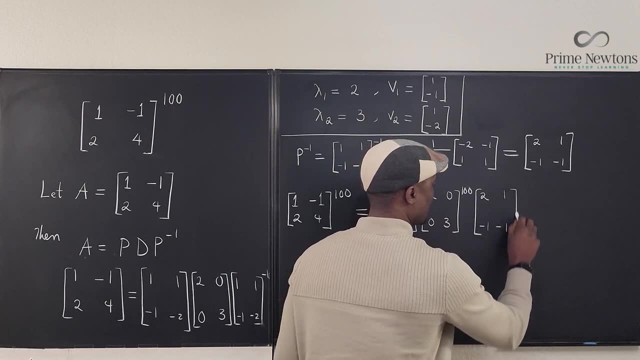 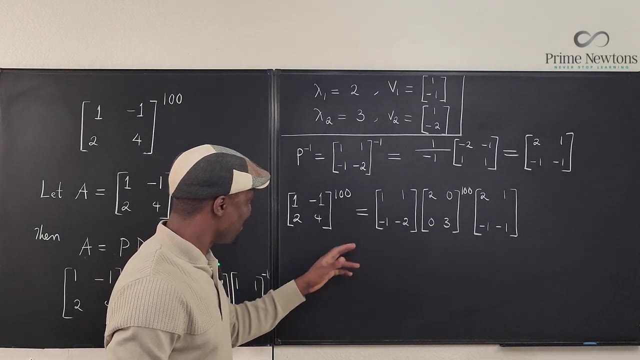 times the inverse, which we just computed: 2, 1, 2, 1, negative, 1, negative 1.. That's what we get Beautiful, Okay, so what happens? Let's compute this. We already know that when we raise this to power, 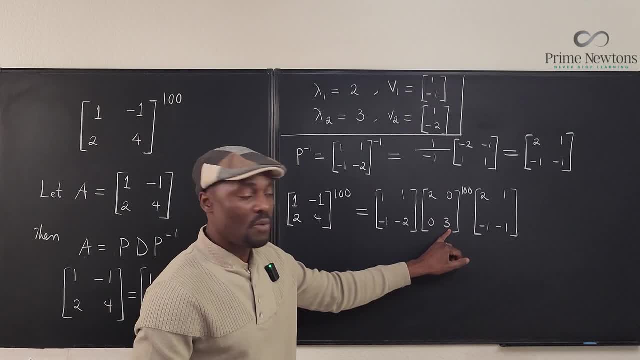 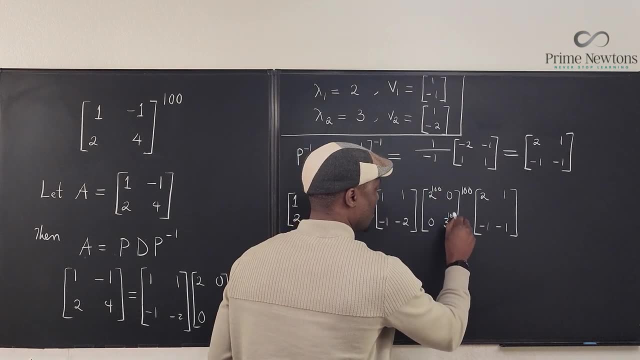 100,. this is raised to power 100,. this is raised to power 100. So I might as well just move it in. So let's write it as 2 raised to power 100, and 3 raised to power 100, and just delete this. 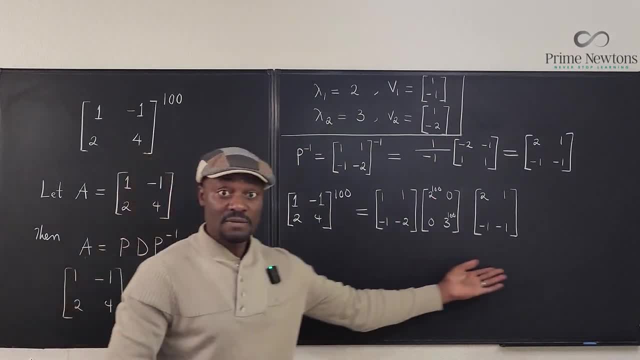 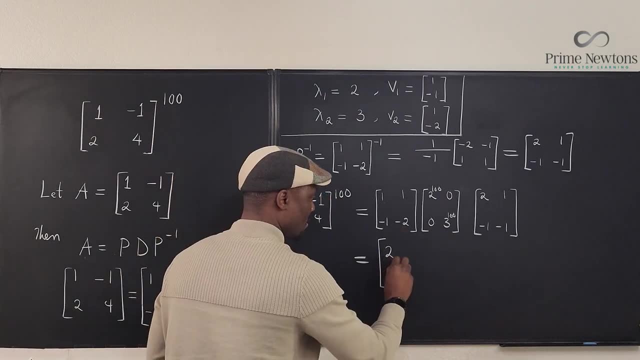 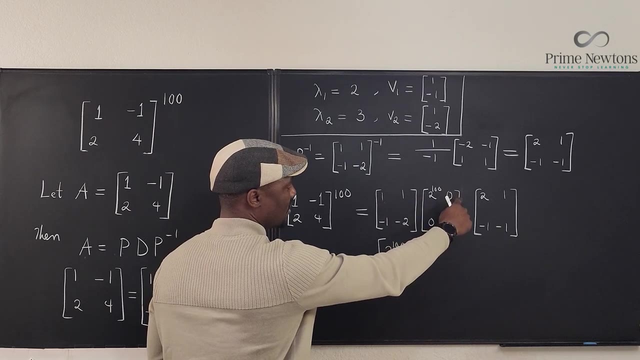 because that's what it means. Okay, so you can leave this as your final answer, depending on what your teacher wants, or you can do the multiplication. Well, let's try and do the multiplication 2 to the 100.. And then, if you take this and multiply this, you're going to get 3 to the 100, to the 100. 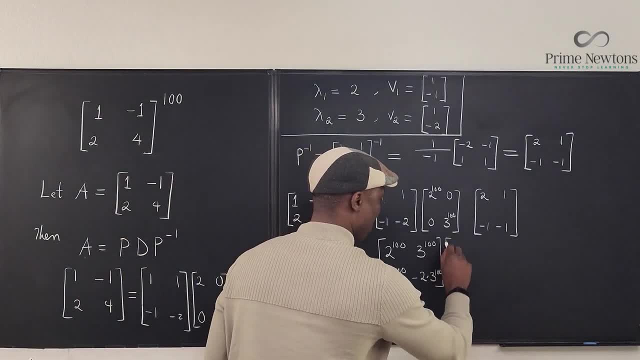 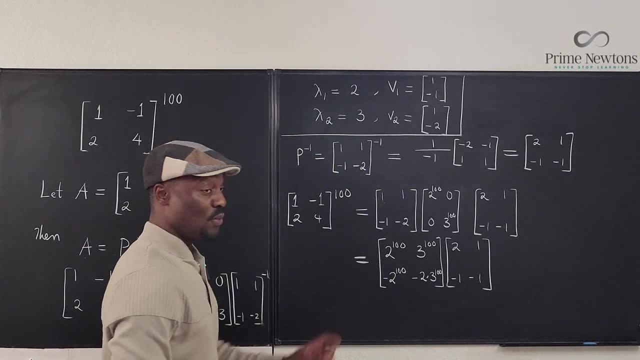 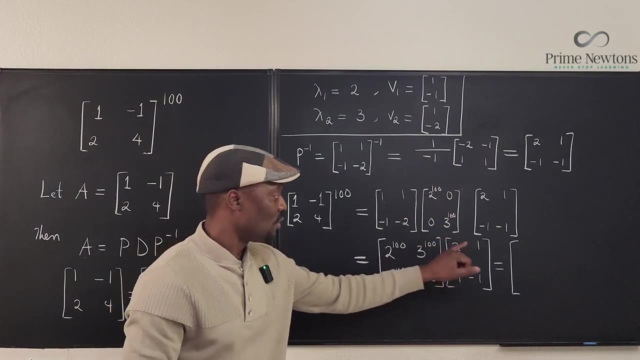 That's what you get multiplied by 2, 1, minus 1, minus 1.. Okay, we're going to do one more multiplication We might need to clean up eventually. Okay, let's see what this is going to give us: 2 to the 100 times 2 to the 1 is going to be 2 to the 101.. 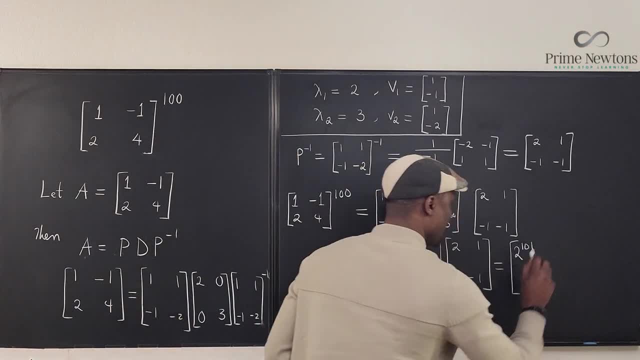 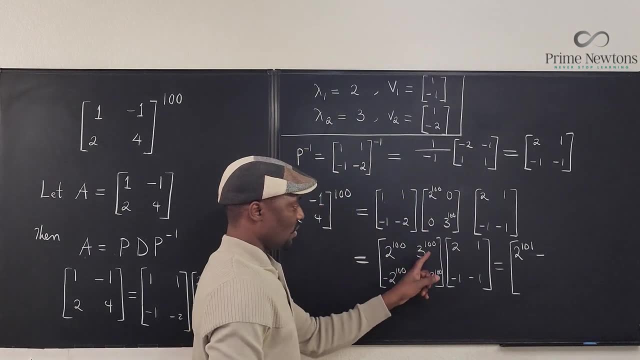 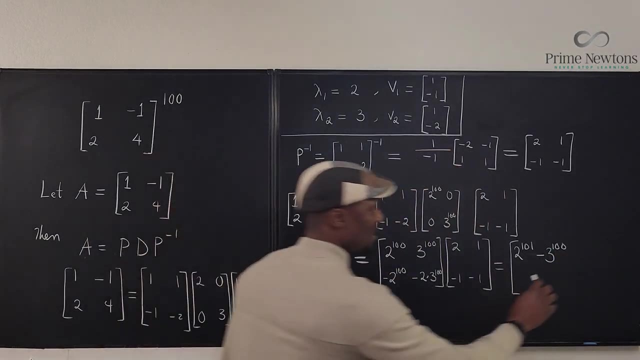 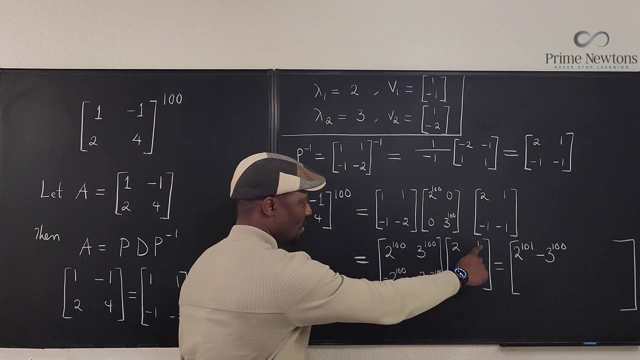 So this is going to be 2 to the 101, rather minus. it's going to be minus 3 to the 100.. That's the first part of the matrix. It's going to be a giant matrix, Okay. and the second part is going to be 2 to the 100. 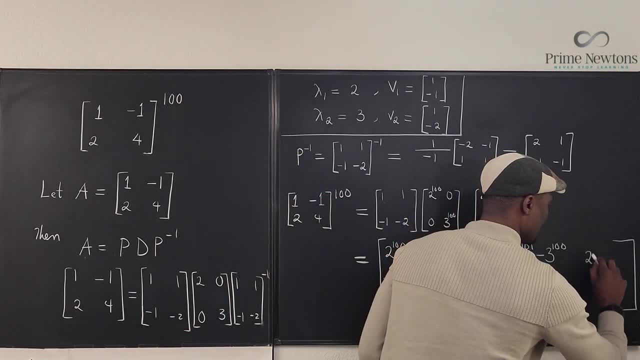 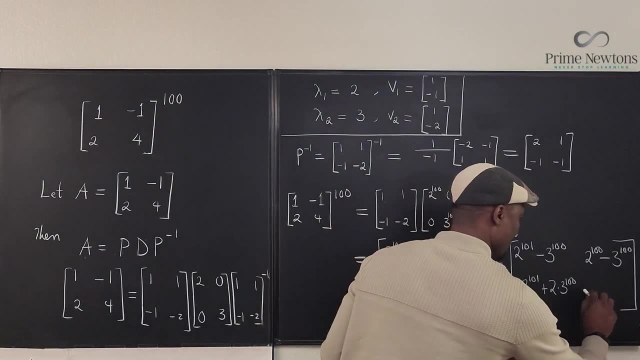 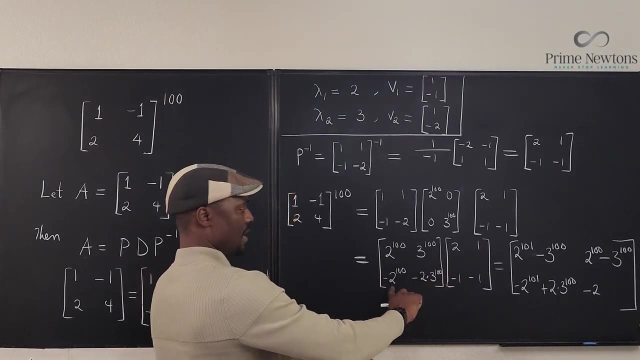 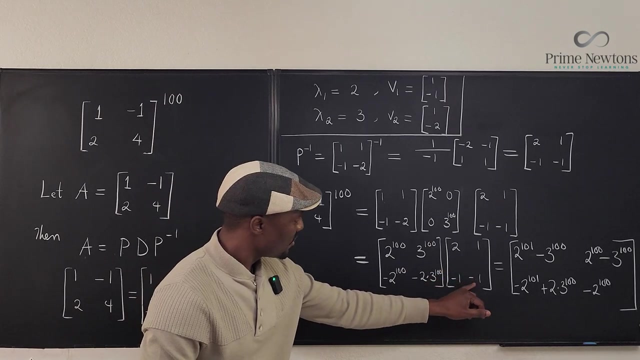 Um, the same thing. it's going to be 2 to the 100 minus 3 to the 100. That's going to be negative: 2 to the negative, 2 to the 100.. Okay, and then the final one is going to be, this times, this, which is going to be plus: